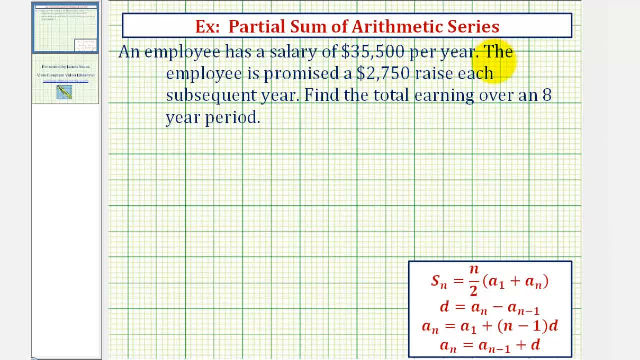 An employee has a salary of $35,500 per year, The employee is promised a $2,750 raise each subsequent year to find the total earnings over an eight year period. So the first thing to recognize about this question is: we're trying to find the total earnings. 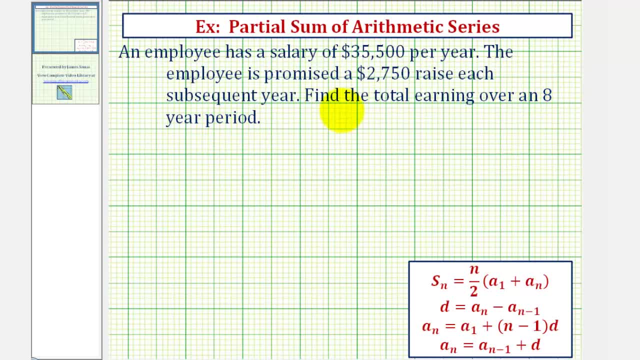 over an eight year period, not just find the salary in the eighth year, And therefore we're finding a partial sum of a series, not a term in a sequence. And because the salary is increasing by $2,750 each year, we're finding a partial sum of an arithmetic series. 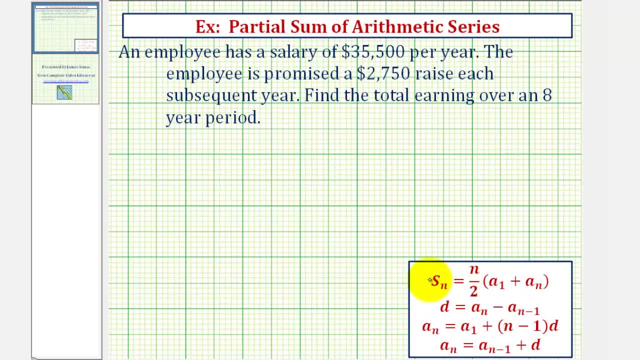 And therefore we'll be using the formulas given here below, where S sub N is the partial sum of the first N terms in an arithmetic series, D is the common difference and A sub N would be the Nth term in the sequence or series. 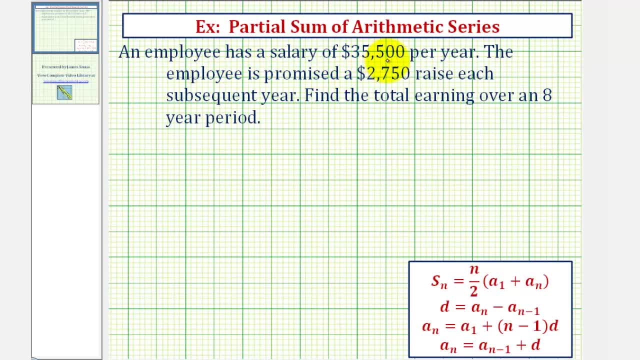 Because the salary of the first year is $35,500, A sub one is $35,500,. the salary is increasing by $2,750 each year and therefore the common difference D is equal to $2,750.. And this is positive because 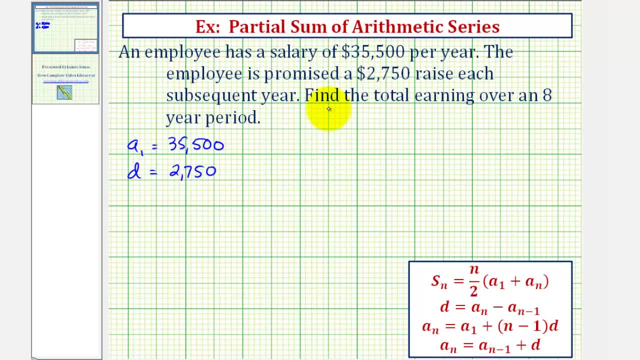 the raise is increasing the salary each year. Our goal is to find the total earnings over an eight year period. so we're trying to find S sub eight, or the sum of the first eight terms in this arithmetic series. And because we're looking for S sub eight, 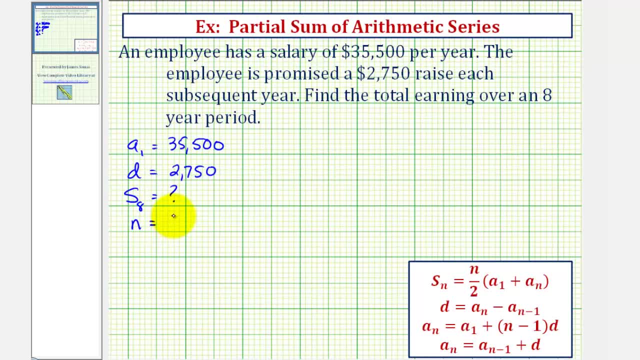 this also tells us N equals eight. Now, if we look at our formulas again, notice how the partial sum formula requires us to have N, which we have, A sub one, which we have, but we don't have A sub N, which in this case would be A sub eight. 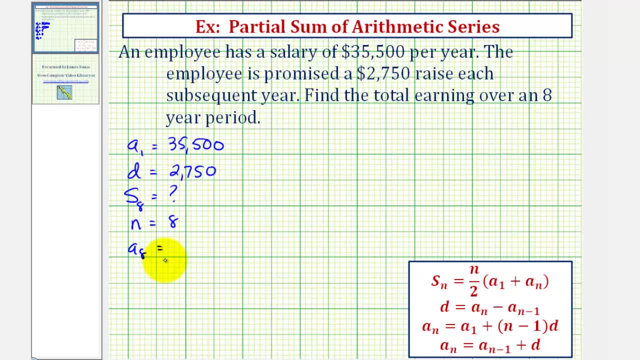 So we'll begin by determining A sub eight and then find the partial sum S sub eight. Notice how there are two formulas for A sub N. but this last formula requires us to have A sub N minus one, or in this case, A sub seven. 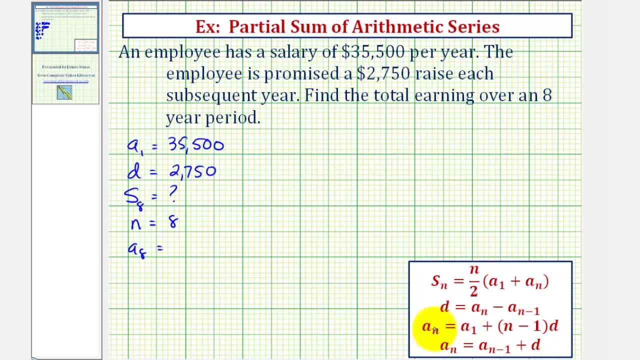 which we don't have. So we'll use this formula here to find A sub eight. A sub eight is equal to A sub one: $35,500, plus the quantity N minus one, that would be eight minus one times the common difference D.